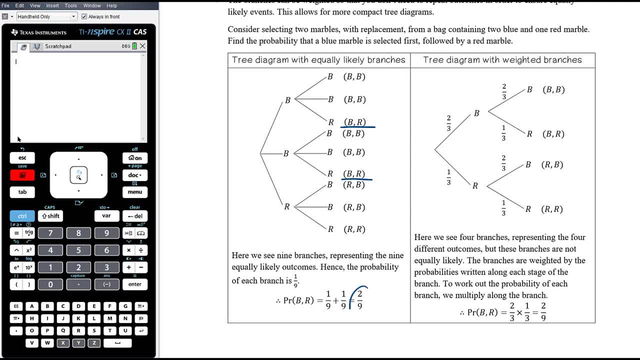 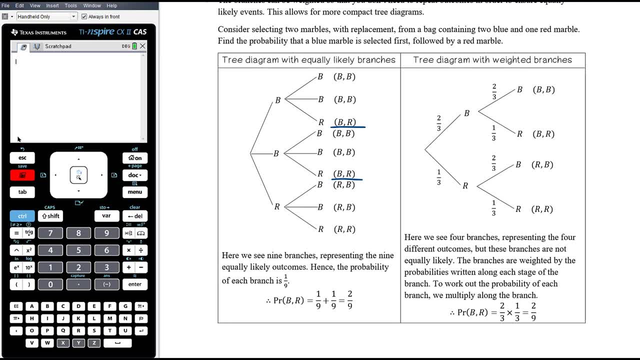 out of the nine, out nine equally likely outcomes, and so two ninths is our probability. We can, however, condense the tree diagram because actually, at each stage, there's only two different things that can happen. We could get a blue or a red marble. okay, so my first choice is: either blue or 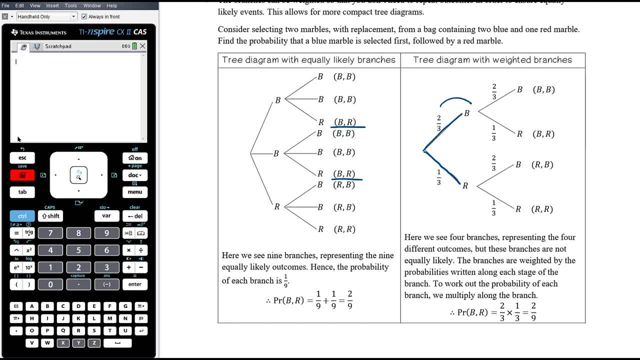 red, but then so it's really important. a lot of students I find jumble these around. okay, so it is two sections. so I start from here, I can then choose blue or red. from there I can then choose blue or red. okay, then I weight the branches of the tree diagram with probabilities, if there's. 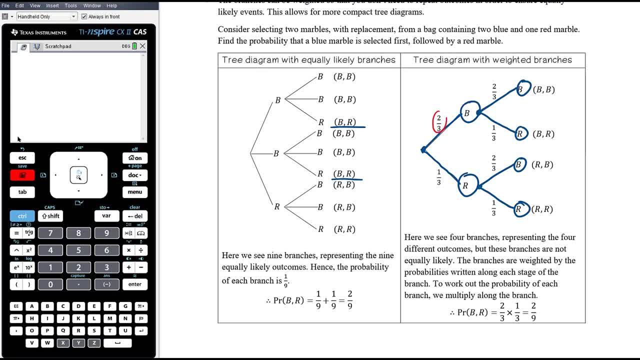 no probabilities in the branches, that means they're equally likely to happen. so on the branch I say: well, okay, but the likelihood of choosing a blue is twice as likely as choosing a red. there's a two out of three chance of choosing a blue and only a one out of three chance of choosing a red. 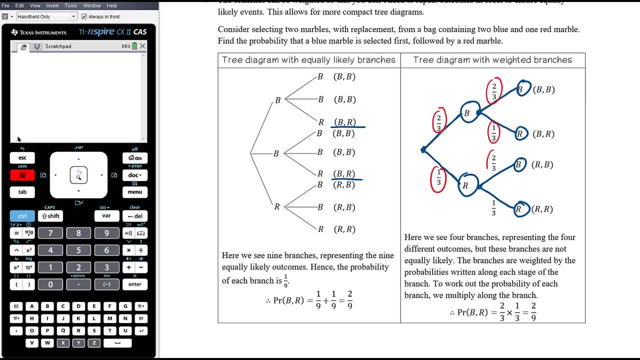 I'm replacing the marble, so there's still a two-thirds and one-thirds chance at the second stage as well. So then, if I want to work out the probability of getting blue and then red, I'm interested in this particular pathway. okay, and when I'm working along a tree diagram, along the branches of a tree diagram, 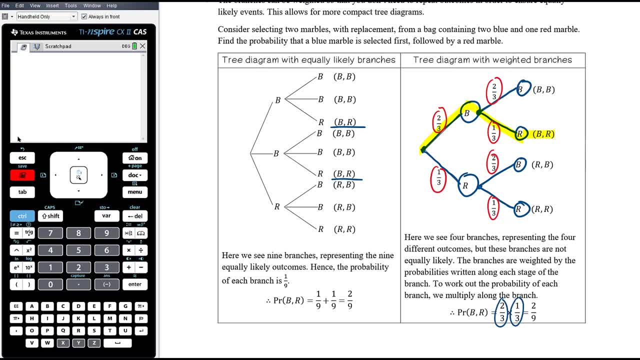 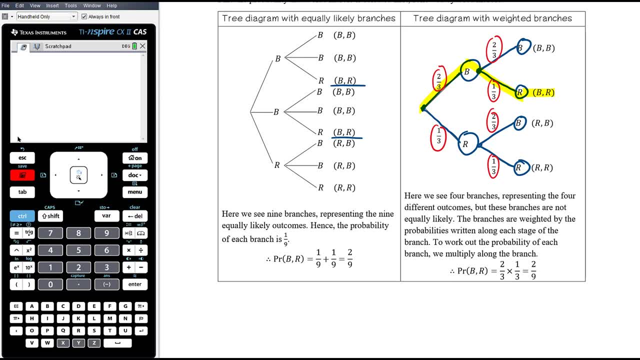 I multiply those probabilities together, so it's going to be two-thirds times one-third, which is equal to two-ninths. okay, so it gives us the same answer. it's the same problem, just formulated in a slightly neater triangle. oh, neater tree diagram, Okay. another advantage is that it's very easy to. 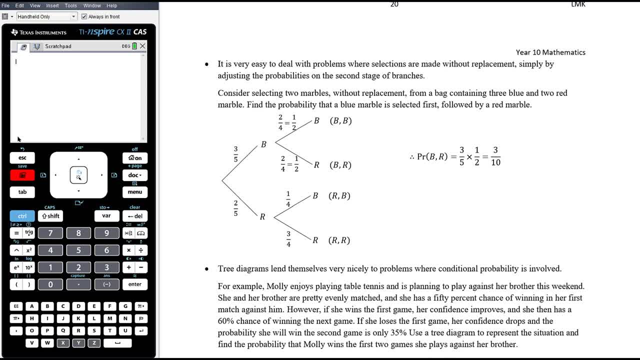 be made without replacement. I'm really not that comfortable doing the tables with that, with the without the replacement. I think it's a bit unwieldy and it's really easy to do that simply by adjusting the probabilities on the second stage of the branches. okay, so if we think about the same, 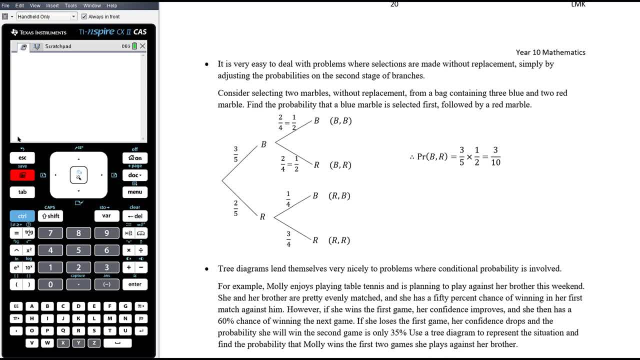 problem. we had before a bag containing three blue and two. sorry, no, it's a different problem. a bag contains three blue and two red marbles. find the probability that a blue marble is selected first, followed by a red marble? okay, so again in terms of setting up the tree diagram, the structure of 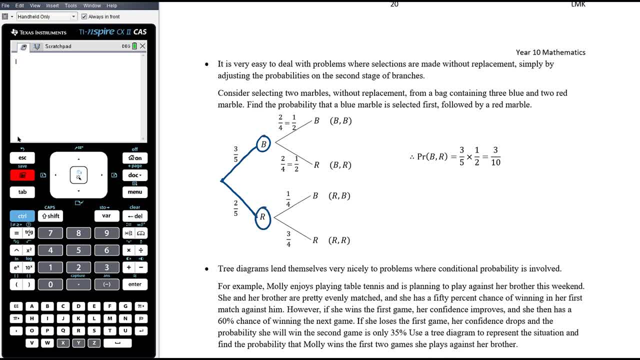 the tree diagram. our first choice involves two options: getting a blue or red and from there. our second choice again involves two options: getting a blue or red. so at the end of the branches is where you list the outcomes. okay, I can get blue and then blue or blue, and then red or red, and then blue or red and then red. those are. 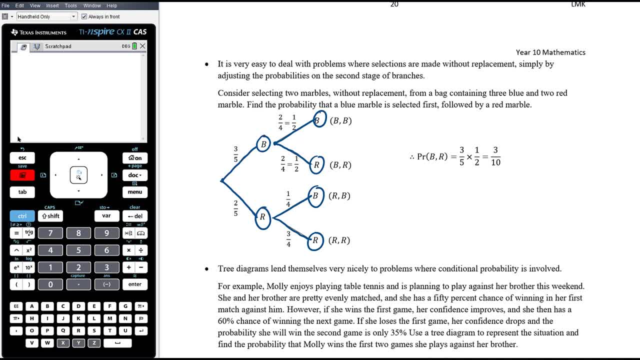 all the options I'm seeing there. then if my branches aren't equally likely, I then weight the branches by putting probabilities on them. so at the first selection I've got five marbles, three then it's without replacement. so if I've drawn a blue marble out of the bag at this point here, the 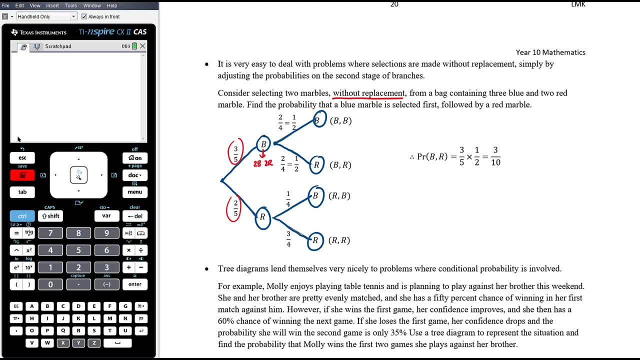 bag now contains two blues and two reds because I've taken out one of these three blues. okay, so I've now got two blues and two reds, which means at the second stage, the probability of drawing a blue is two out of four or a half, and the probability of drawing a red is two out of four. 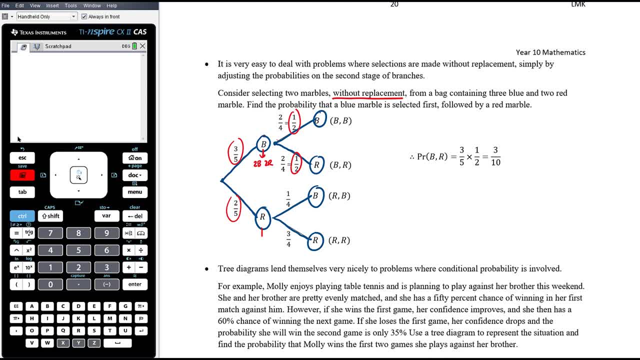 or a half. okay, if I drew a red marble first, what I have left in the bag is three blues and one red. so then the probability at the next stage of choosing a blue is: um, oh, sorry, I've got those around the wrong way, haven't I? can we correct that? sorry, that's a three quarters chance of. 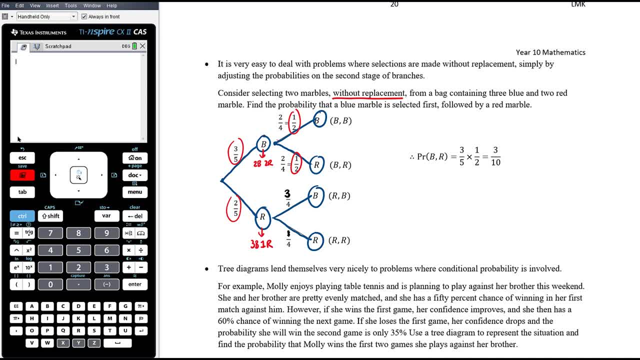 getting a blue and a one quarter chance of getting a red. okay, um, so you, you just think carefully about what's happening at that second stage. and then the probability of getting a blue and then a red. the branch that I'm interested in is blue and then red, so I multiply those probabilities together three-fifths times one-half, and that is. 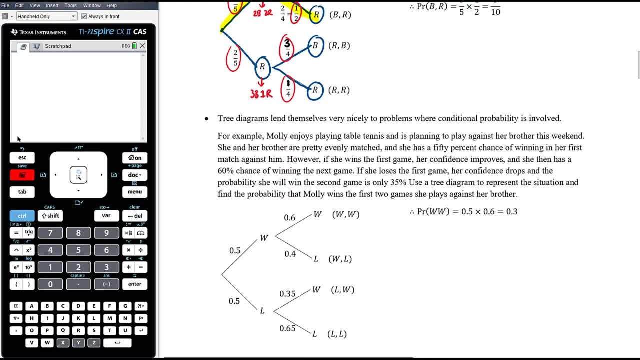 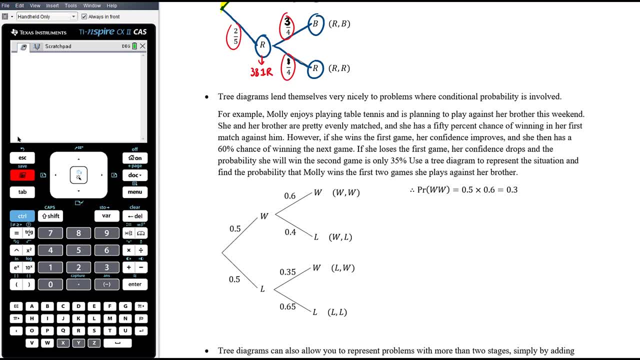 three-tenths. the other advantage is that tree diagrams lend themselves very nicely to problems where conditional probability is involved. so if you're given conditional probabilities as part of the description of the problem, absolutely that screams. please use a tree diagram. okay, because actually in the tree diagram the second stage of the branches, the probabilities here, this second. 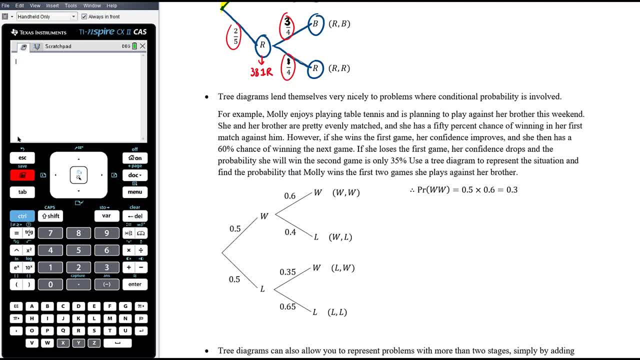 stage. they are all conditional probabilities, okay, um. so let's have a look at the description first, and then I'll talk through that conditional probability thing a bit more. so Molly enjoys playing table tennis and is planning to play against her brother this weekend. she and her brother are pretty evenly matched and she has 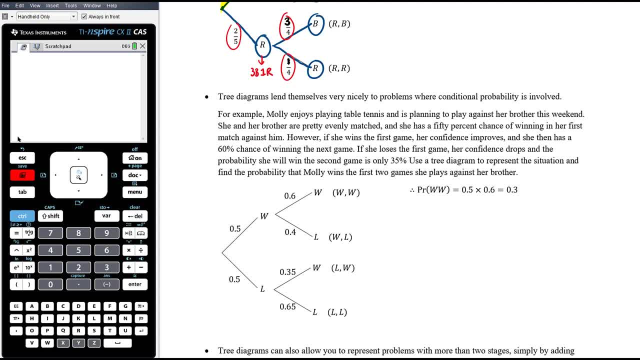 a 50 chance of winning in her first match against him. however, if she wins the first game, her confidence improves and she then has a 60 chance of winning the next game. if she loses the first game, her confidence drops and the probability she will win the second game is only 35. 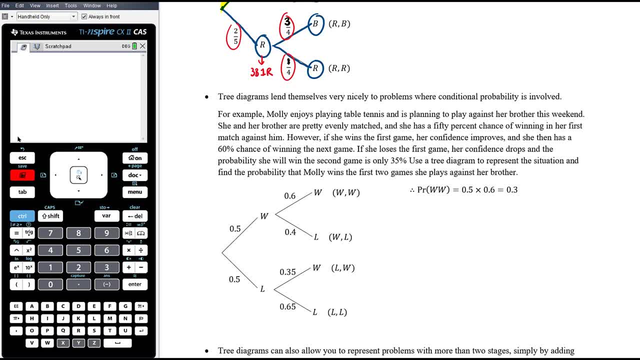 use a tree diagram to represent the situation and find the probability that Molly wins the first two games that she plays against her brother. so in this question we're actually given two conditional probabilities. this 60 and this 35 are both conditional probabilities. the 60 is the probability. 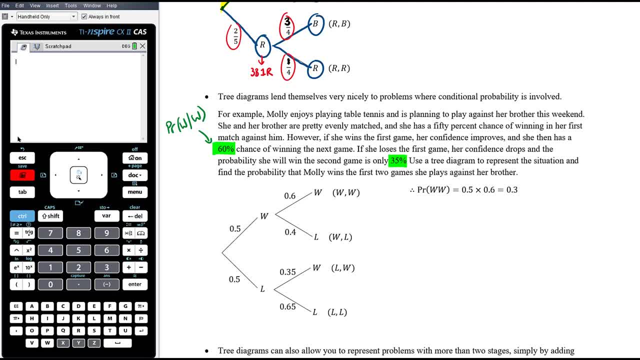 that she'll win the second game, given that she won the first game. and this probability is the probability that she'll win the second game, given that she lost the first game. okay, and we are seeing all four probabilities here at the second stage are conditional probabilities. this point four then. 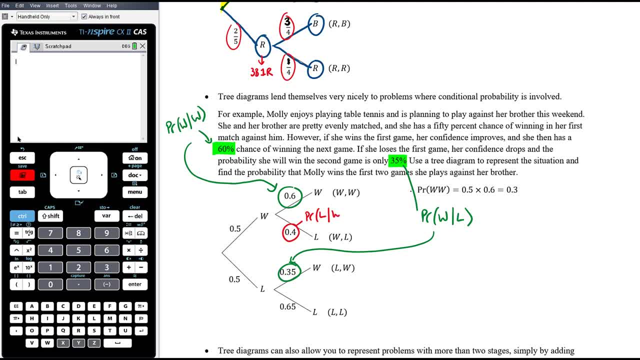 is the probability that she loses the second game, given she won the first game. and this is the probability that she loses the second game, given that she lost the first game. so we've got four conditional probabilities at that second stage of the trader tree diagram. so if part of 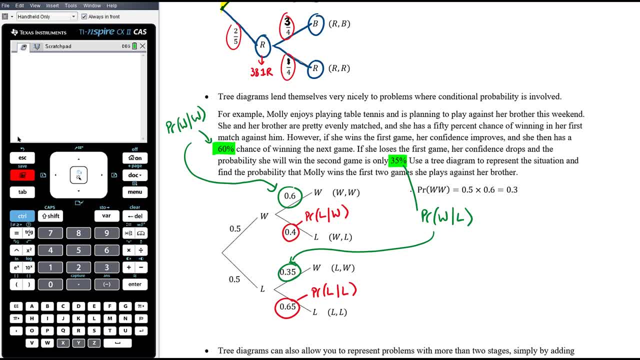 the information. your question is a conditional probability. a tree diagram is going to be key. and then the question is: what is the probability she wins the first two games she plays against her brother? so we want probability of win and then win okay, and so that is going to be 0.5 times 0.6, which 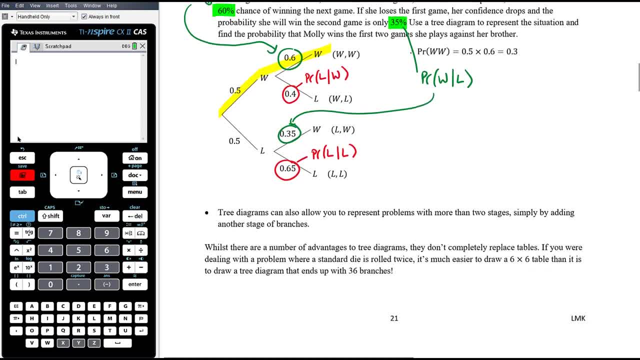 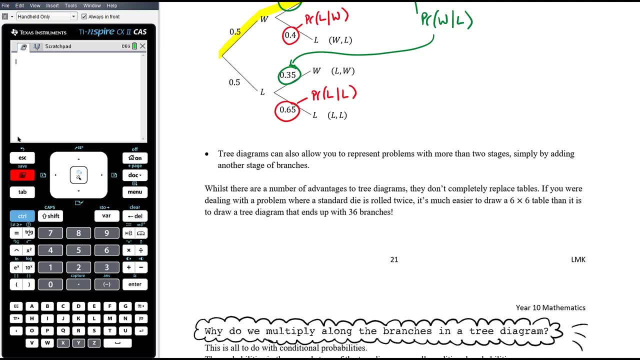 is 0.3. tree diagrams can also allow us to allow us to represent probability problems with more than two stages, simply by adding another stage of. so if they were to play a third game, she could win and then lose, win and then lose, Etc again. okay, so with that's a limitation of a table, we could only 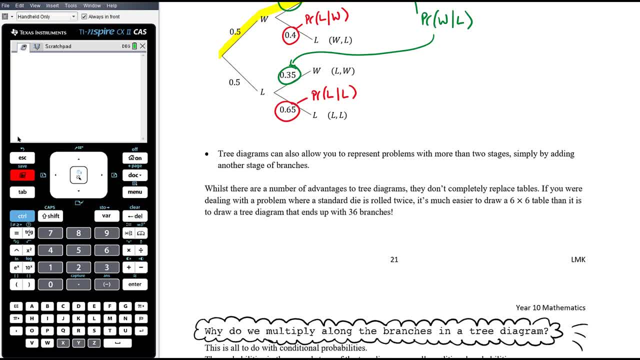 have two stages. so whilst there are a number of advantages to tree diagram- tree diagrams, which I've listed above- they don't completely replace tables and if you were dealing with a problem where a standard die is rolled twice, it's much easier to draw a six by six table. I know that's a bit tedious than it is. 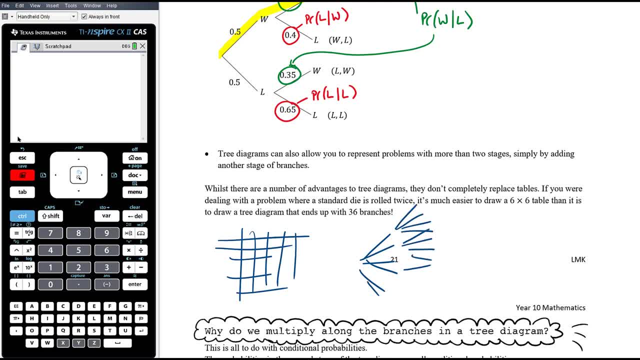 to do a six branches and then six branches. you have a tree diagram with 36 branches. okay, so there are pros and cons to both. I would say, more often than not, a tree diagram is the best way to go, but absolutely, there are examples, as such as the one mentioned here, where a table actually is. 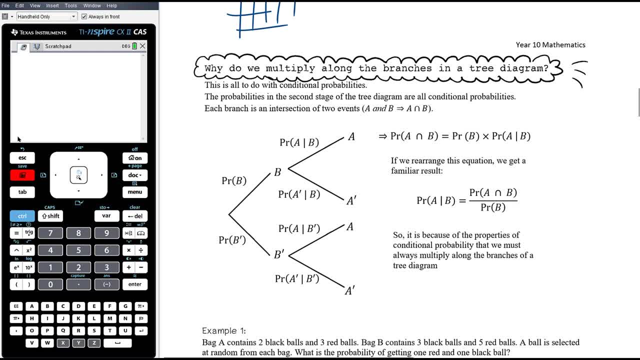 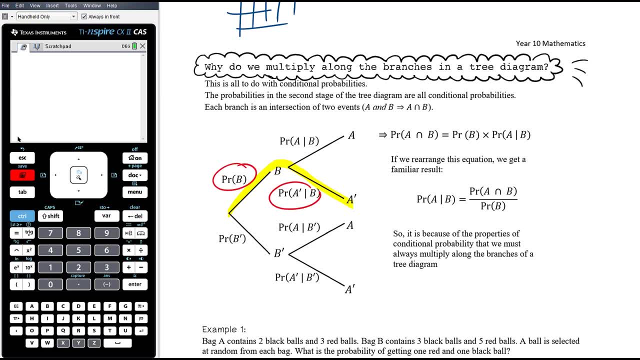 high in level variance, so it's really we're going to have to pick out the correct number to be built down in big picture. second, to somerset, these will all sort of overlap into elements now because it's a reduction in the number, so I'll be using these to more Mahler and Gal. 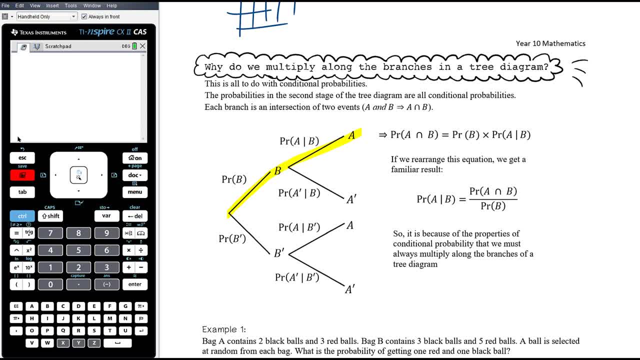 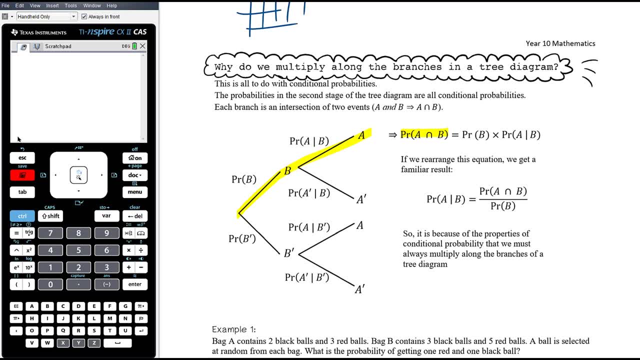 is out of the running verb, so Z cash is out of the row, so we'll we'll have to take that with us over to three V, then we can go back to the please'm separate unit. So that was a, just to show us a little work out probability of A intersection B, And we know from what we've been doing so. 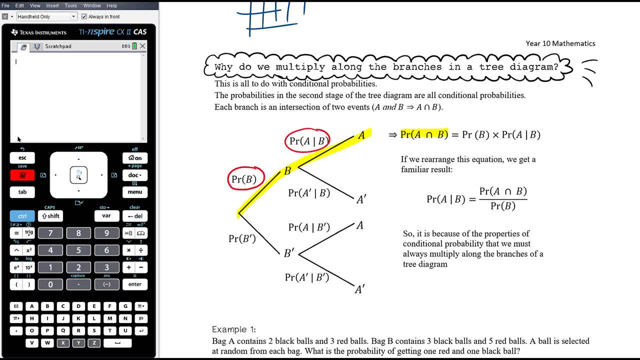 far. I've told you that you need to multiply these two probabilities together in order to get the probability of A intersection B. So probability of A intersection B is probability B times the probability of A given B. If we then rearrange this equation, so divide both. 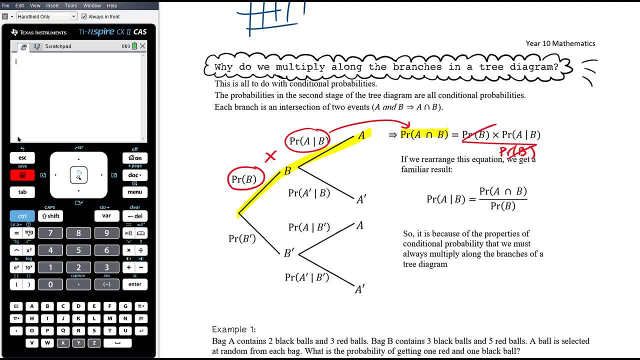 sides by B, which cancels it out from here and puts it over here, we get this: Probability of A given B is the probability of A intersection B over the probability of B. So the fact that we multiply the probabilities along the branches is all to do with our understanding of how. 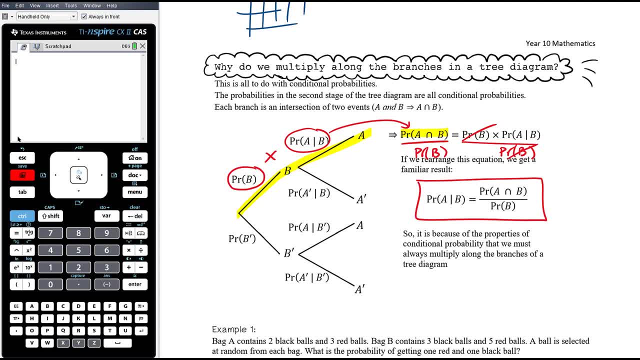 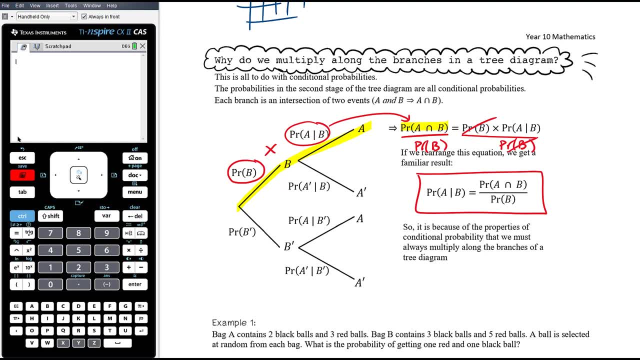 conditional probability works. So that's why we always multiply along the branches If we're interested in more than one branch. so if we actually want to know the probability of A intersection B, or the probability of A intersection not B, we would then multiply. 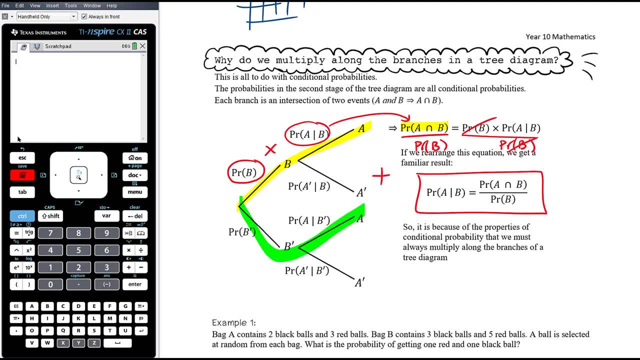 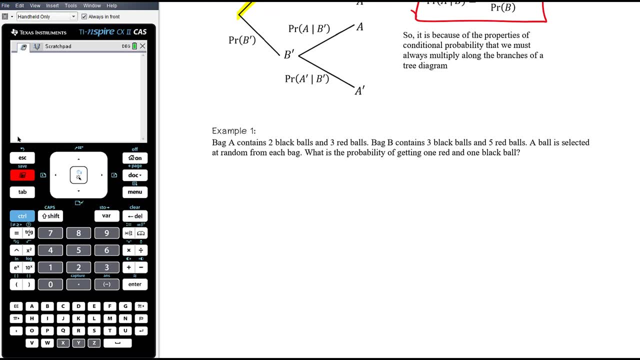 along the two different branches and then we would add- We'd add- that probability together. Let's have a look at some examples. Bag A contains two black balls and three red balls. Bag B contains three black balls and five red balls. A ball is selected at random from. 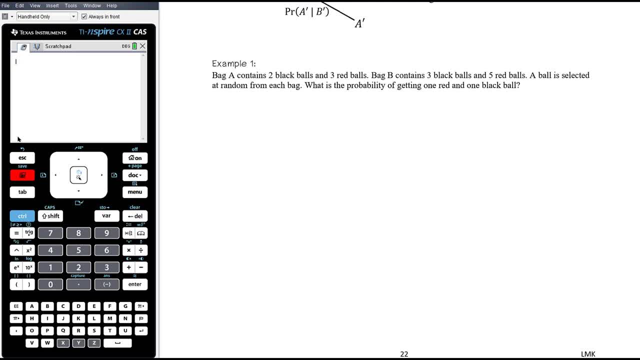 each bag. What is the probability of getting one red and one black? It's really important that you read the question carefully here. This question could also have said: a bag is selected first and then a ball is selected. Then you draw a different tree diagram, but in this case it is a ball is selected from. 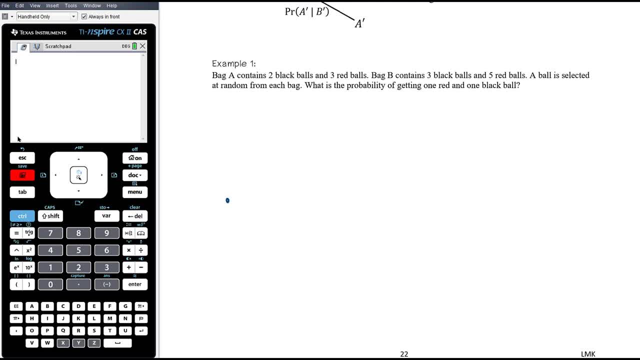 each bag. Our first selection is going to be from bag A, and the options that we could get from bag A would be a black or a red Advise with a tree diagram. Always start with quite wide branches to give you room to be able to extend from each of them. 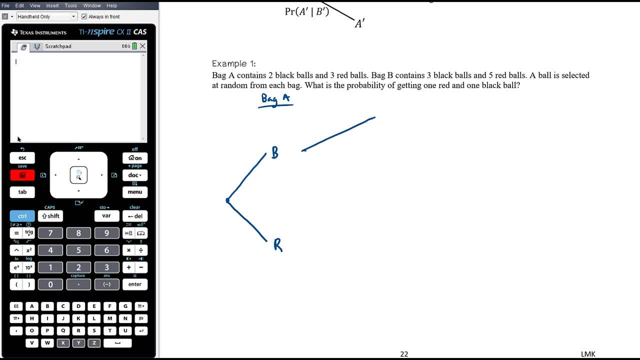 Bag B contains three black and five red. Again, in terms of outcomes, we could get black or red, Black or red. Yes, Yes, they're not equally likely, so we'll weight the branches bag B. okay, so that's our two stages, our. 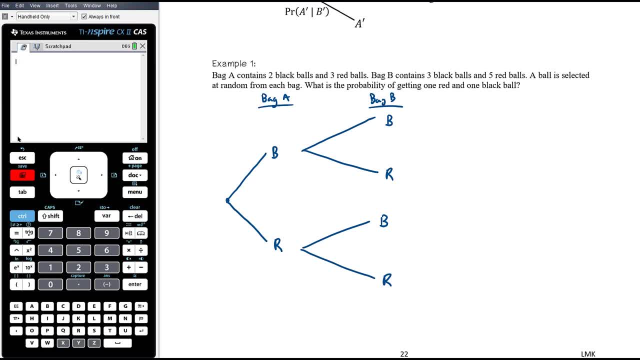 two selections, the outcomes that are possible. now we want to weight the branches with the probabilities. okay, so when we're selecting from bag A, the probability will select a black ball. we've got three out of eight balls are black and five out of eight balls are red. then when we 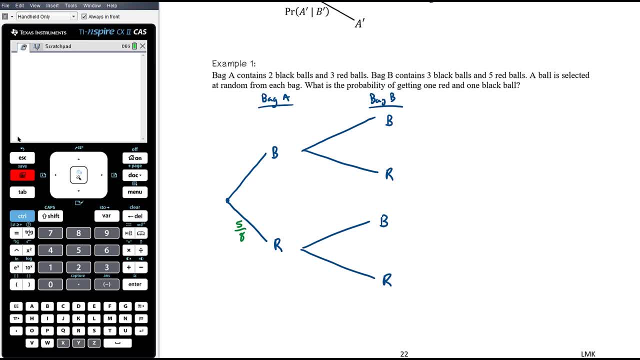 select from bag B. bag B: oh sorry, I did bag B first. I read the wrong bit. sorry bag, sorry. bag A contains two black and three red. okay, so it's: two out of five are black and three out of five are red. and then, when we make our selection from bag B, we've got three out of eight are black. 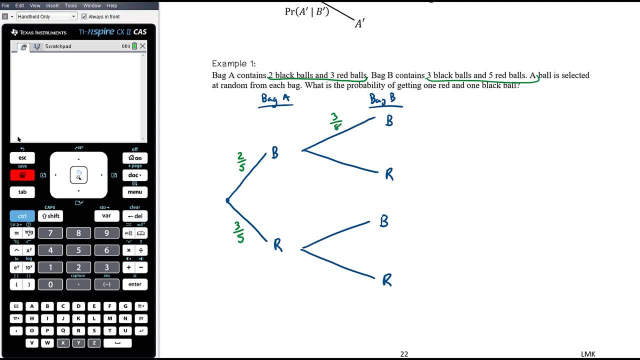 three out of sorry, five out of eight are red, three out of eight are black and five out of eight are red. it's really important. it's really important that when you draw a tree diagram, if you add up all the probabilities that stem from the one point. 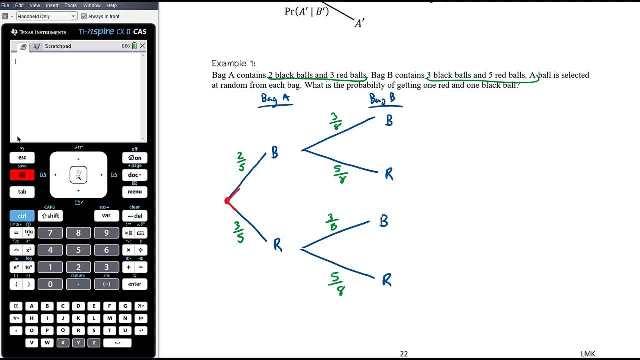 the two-fifths plus three-fifths must add to one. if they don't add to one, there's a third branch here that you've missed, okay, so it's really important that if all the probabilities are stemming from the one point, they must add to one. three-eighths plus five-eighths is one. 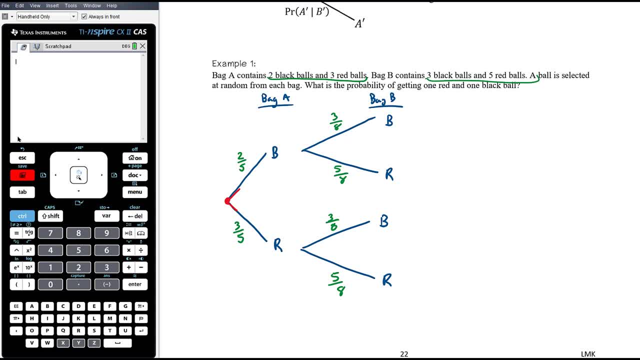 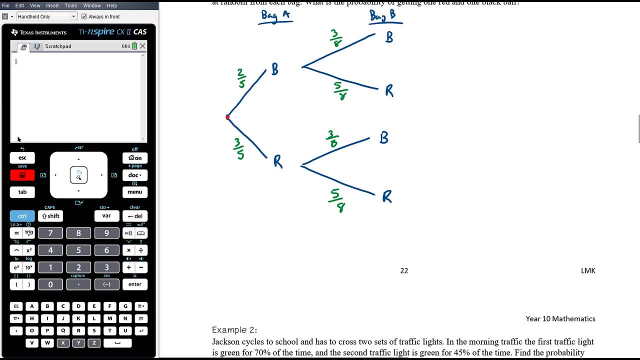 and so that's all good from there. okay, all right. so the question we want is the probability of getting one red and one black. okay, probability of one red, one red, one black. sorry, there are two ways that can happen. you could get a black and then a red, or we could get 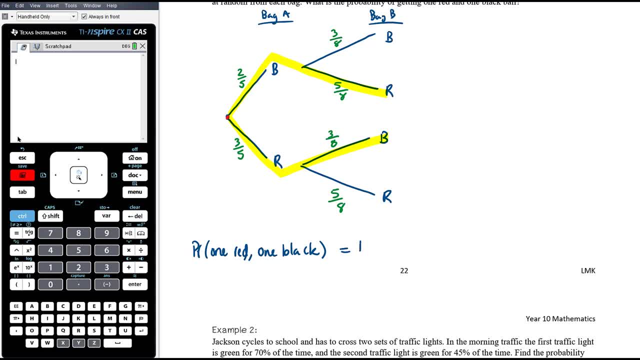 a red and then a black. okay, so probability of black and red, or probability of red and black when we would use the word or, sorry, we add. talk more about that later on in the counting method. okay, so black and then red is two-fifths times five-eighths plus red, and then black is three-fifths. 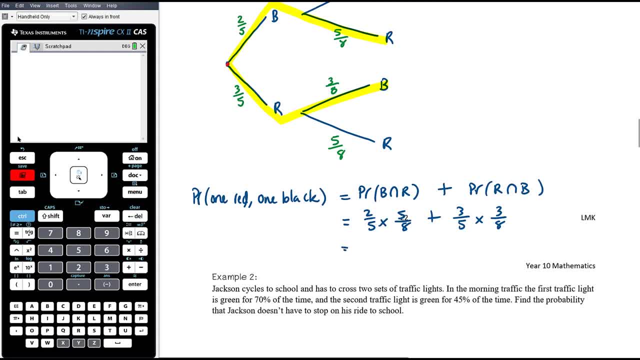 times three-eighths. okay, now we could. I would normally simplify these fractions here and then multiply them together, but if I do that then I'll have a not common denominator for the adding, so I'm going to just leave them as they are, just multiply along. so it's 10 on 40, which, yes, would. 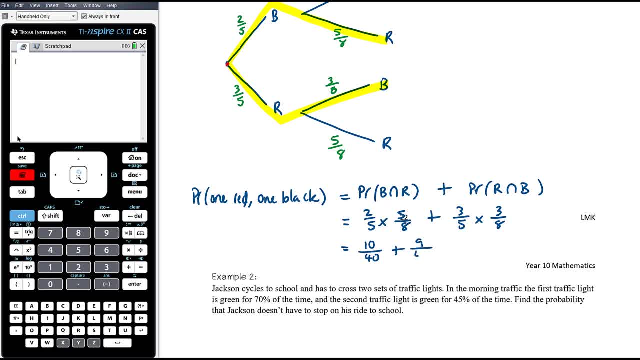 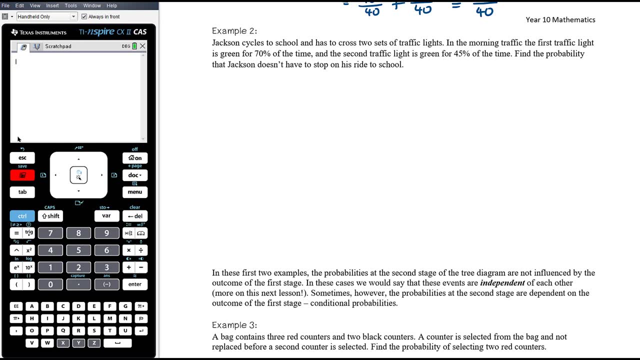 simplify to a quarter, but it's not helpful given that I'm going to want to add it on to 9 on 40. let's keep the common denominator. so it is 19 on 40, so just less than half the probability that I would draw one of each color. all right. example: two Jackson cycles to school and has to cross two. 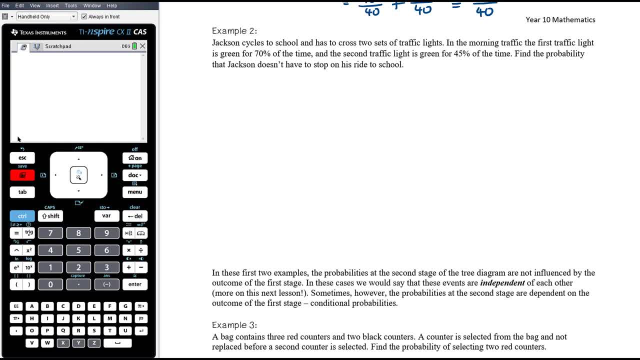 different, sorry, two sets of traffic lights in the morning traffic. the first traffic light is green for 70 percent of the time and the second traffic light is green for 45 percent of the time. find the probability that Jackson doesn't have to stop on his ride to school. okay, so the two stages of the 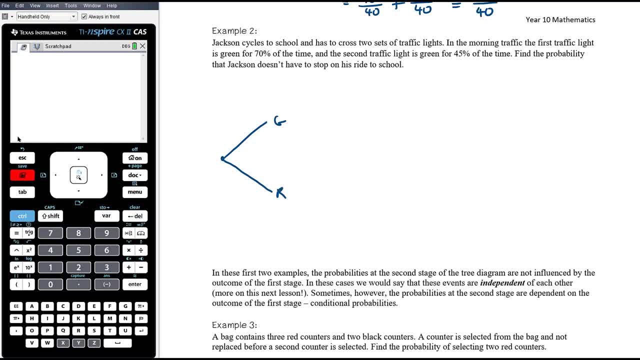 traffic lights and at each traffic light it could either be green or red, green or red. okay, so the probability of a green light at the first traffic light is 0.7 and red is 0.3. probability of a green traffic light at the second traffic light is 0.45, so the red is 0.55. 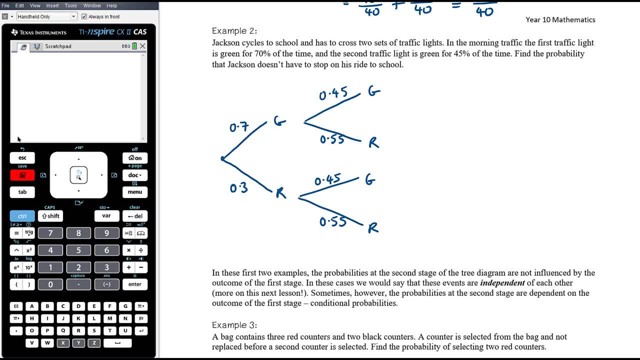 okay, so that's what could happen. we want the probability that he doesn't have to stop, so that is the probability that he gets green and green. so that's going to be working our way along here. so that is going to be 0.7 times 0.45. just going to get my guys to do that for me. 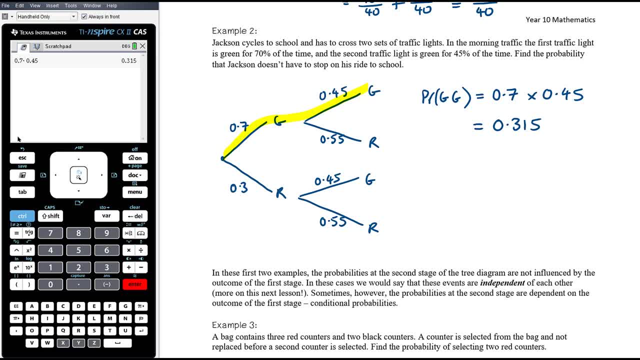 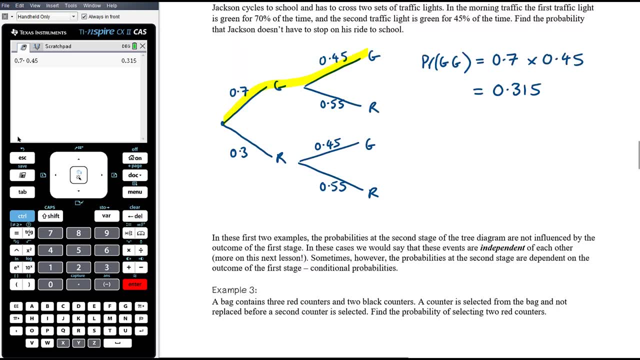 0.315. you could do 7 times 45, 7 times 40 is 28 and 7 times 5 is 35. 28 plus 35 is 315, and so therefore, that's where we get the 0.315. okay, in these first two examples, the probability at the second stage of the tree diagram are not. 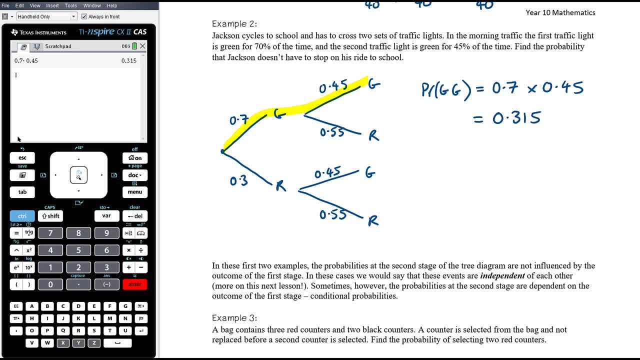 influenced by the outcome of the first stage. in these cases, we would say that these events are independent of each other. we'll talk about that more in the next lesson. sometimes, however, the probabilities. so what we're talking about here is the fact that this, the probability of, 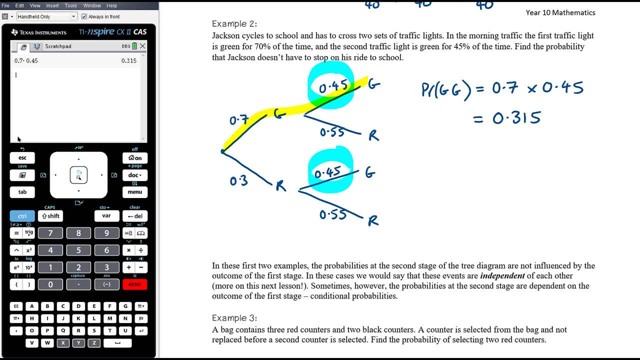 a green light at the second traffic light didn't change depending on whether there was a green light at the first traffic light. they were completely independent of each other. it's, by definition, the idea of an independent event. as i said, we'll talk about more that more in the next video. 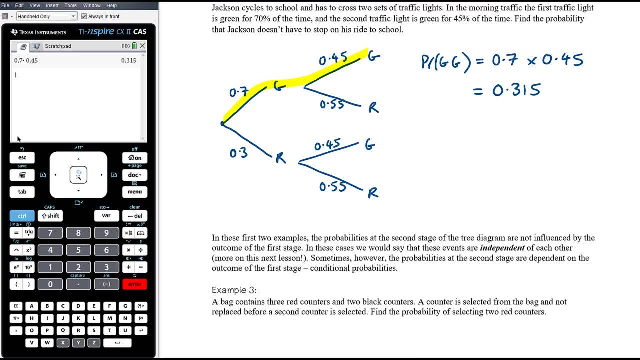 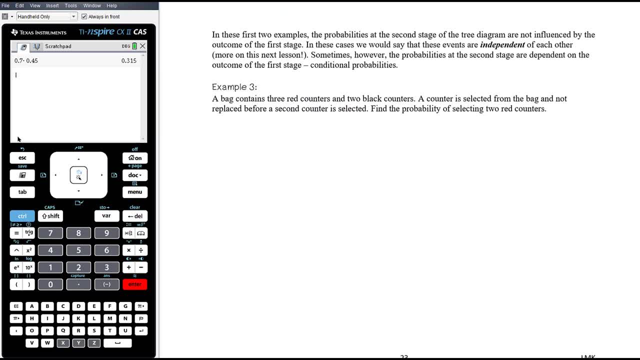 sometimes, however, the probabilities at the second stage are dependent on the outcome of the first stage, and that's when they're conditional probabilities. so let's have a look at some examples where that happens. a bag contains three red counters and two black counters. a counter is selected from the bag and not replaced before a second counter is selected. find the probability. 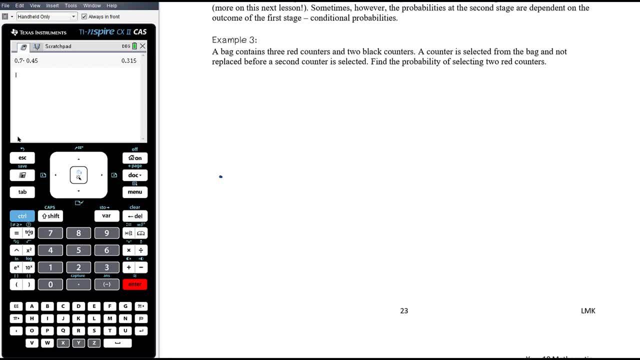 of selecting two red counters. okay, so this time it's not two different bags, it's just two selections from the same bag. but it's still two stages. at our first selection, we could get a red or a black counter. at our second selection, we could again get a red or a black counter. 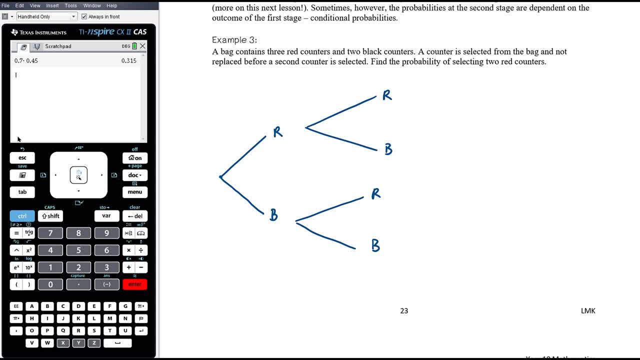 okay, it's got three red counters and two black counters. so therefore, at our first selection, the probability that we get a red counter is three out of five and the probability that we get a black counter is two out of five. okay, then we need to think about the conditional probabilities at the second stage. so if we draw out a red counter, 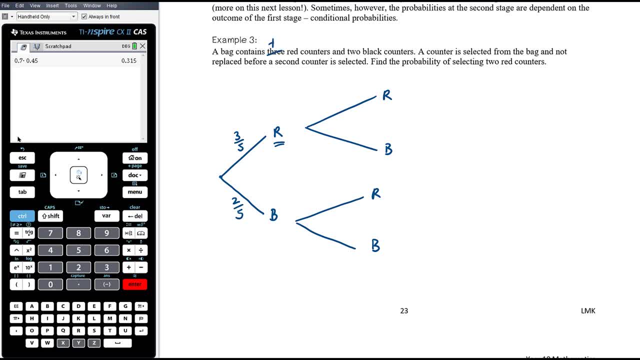 first, okay. then when we, if we take out a red counter, we now only have two red and two black. so the probability of getting a red at the second selection is two out of four, which is a half. probability of getting a black is two out of sorry four, which is a half. alternatively, if we drew a 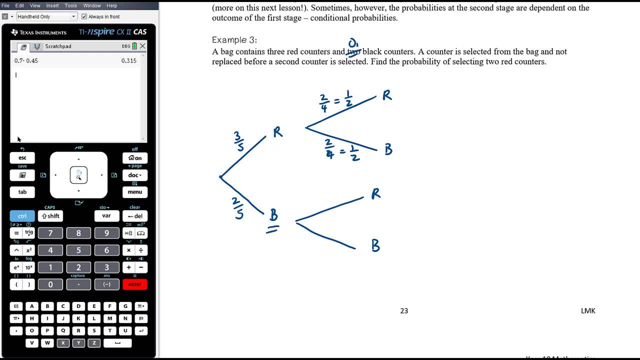 black counter. first we would still have three red counters and only one black counter, so the probability of selecting a red counter at the second selection would now be three out of four, and the probability of selecting a black counter would be one out of four. okay, so then we want the probability of selecting two reds, so the probability of getting red and 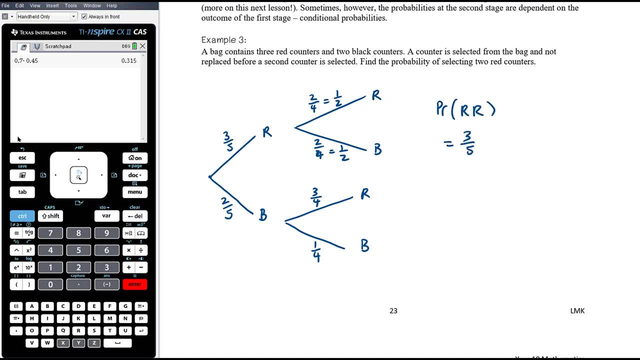 then red is going to be three fifths times one half, which is um three on ten. that's a fraction in simplest form, or you can write it as point three if you really want. there's absolutely nothing wrong with three tenths. just leave it as three tenths. 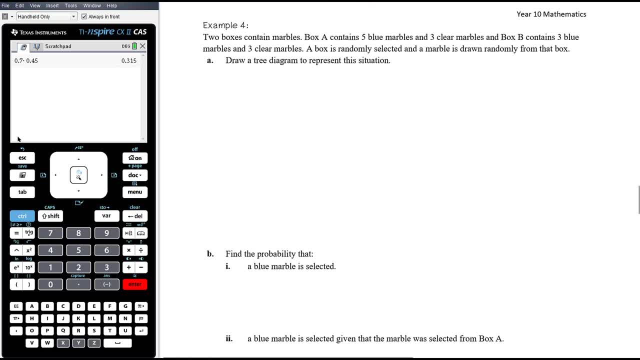 okay. question four: two boxes contain marbles. box a contains five blue marbles and three clear marbles. box b contains three blue marbles and three clear marbles. a box is randomly selected and a marble is drawn randomly from that box. so this is where it's really important that you 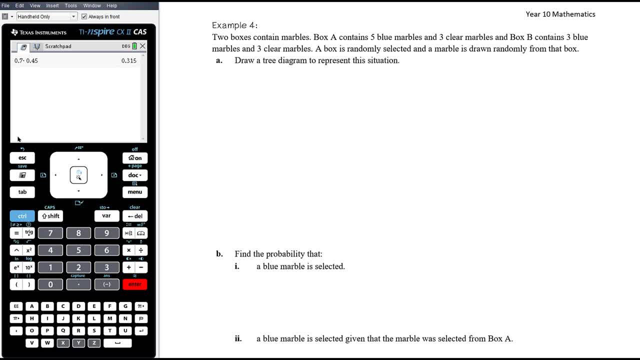 read the question carefully. okay, this time we're not selecting a marble from each box. we are first selecting a box and then we are selecting a marble from that box. okay, so in this case our first selection isn't blue or clear. our first selection is either box a or box b. 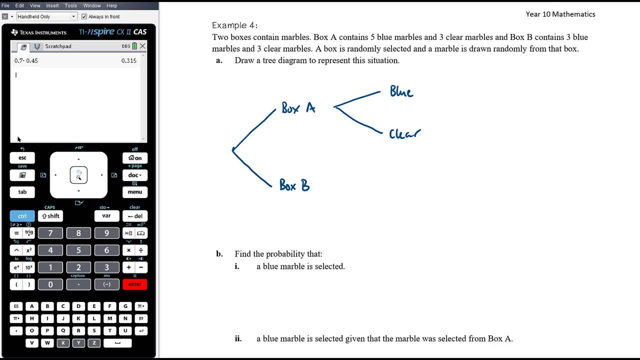 and then from box a we could choose a blue or a clear marble, and then from box b we could choose a blue or a clear marble. okay, again, we want to wait with probabilities. so it says a box is randomly selected. so there are two boxes, we randomly select one, which means each has an. 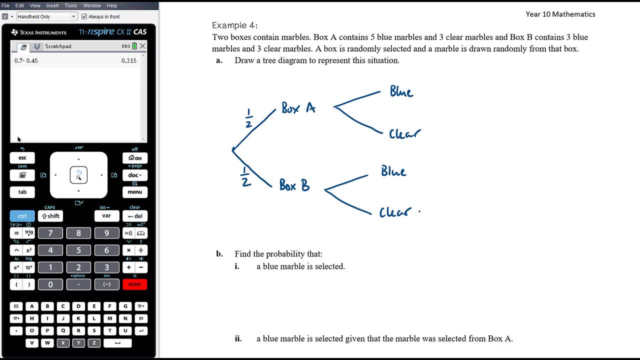 equally likely chance of being selected, so that's half and half. then, if we choose box a, box a as has three clear marbles, so we have a five eighths chance of choosing a blue marble and a three eighths chance of choosing a clear marble. if we choose box b, it has three blue and three clear. 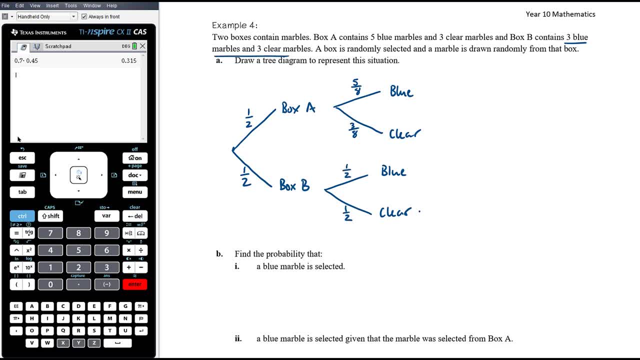 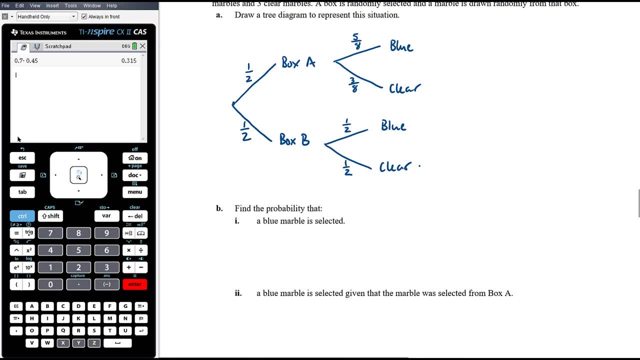 so that is three out of six or half, and three out of six or half, um, okay, so then. so part a: draw a tree diagram to represent the situation. so we've done that. part b: find the probability that a blue marble is selected. so, probability, we get a blue. now there's two ways to get a blue. 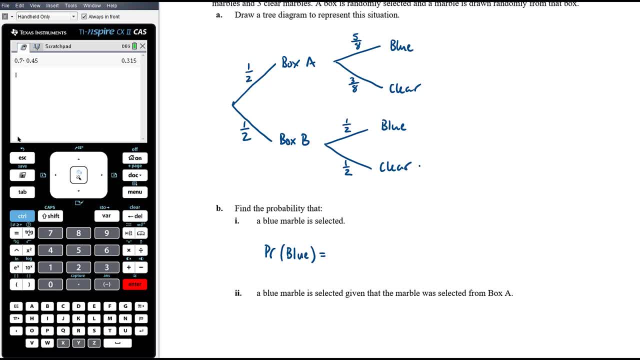 uh, so just going to make, just going to move that up a little, there's two ways to get a blue. that would be probability of getting sorry box a, choosing box a and a blue marble, or the probability of choosing box b and a blue marble. okay, so essentially it is this branch. 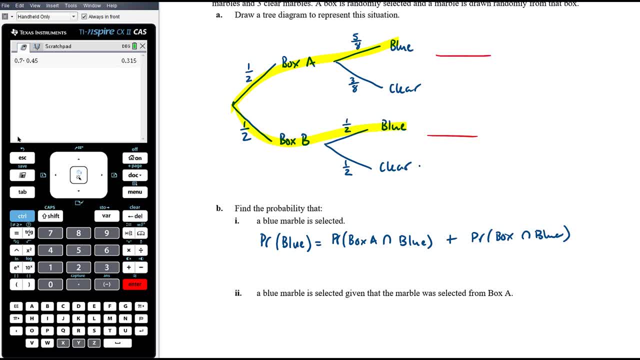 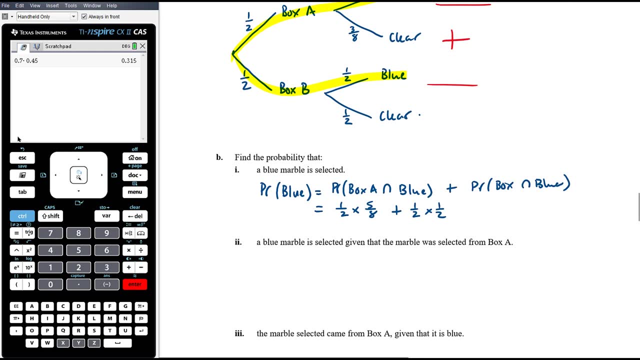 plus this branch. okay, so we work at this probability and we add: okay, so the probability is the probability of choosing box a and a blue marble is half times five, eighths, plus choosing a blue marble from box b is half times half. okay, and so that is five on sixteen plus one quarter, which is five on sixteen plus. 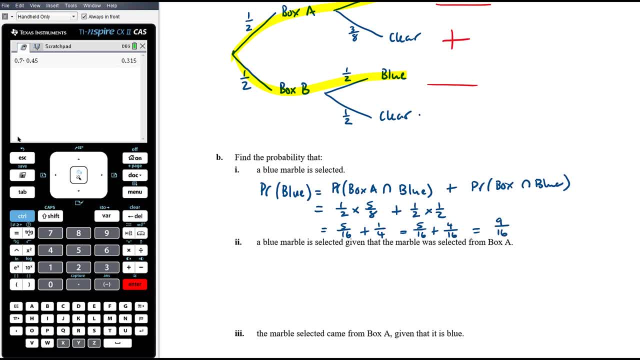 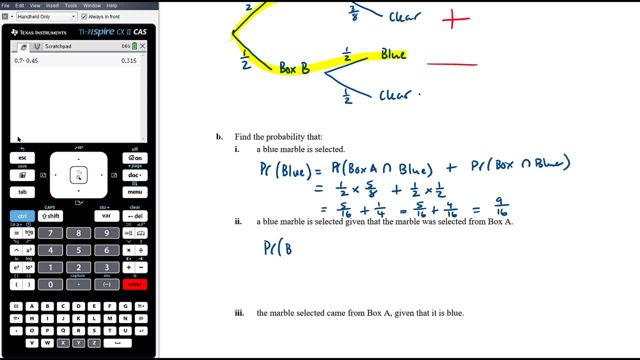 four on sixteen and so that is nine on sixteen. part two find the probability that a blue marble is selected, given that the marble was selected from box a. so probability 17 is said is probability of blue, given it came from box A. Now this is in the tree diagram. that's here. 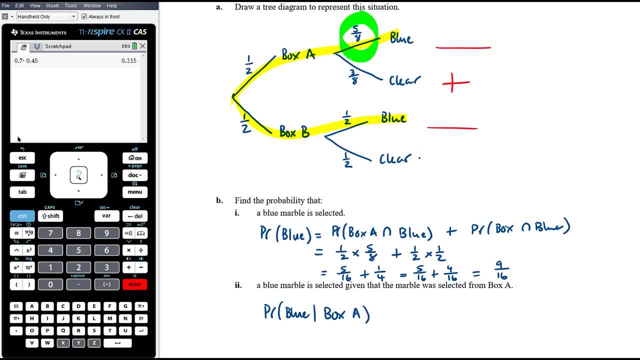 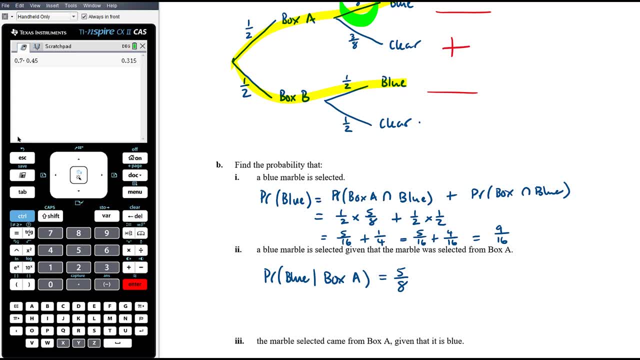 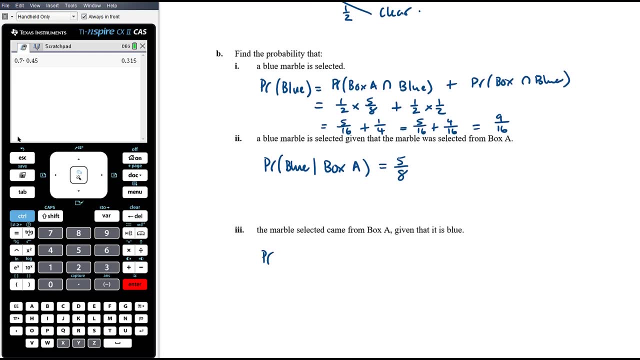 probability we choose a blue marble, given that it came from box A. that's just sitting there. that's five-eighths. that's exactly what that branch represents. probability of giving choosing a blue marble, given that we chose box A. Then we want the probability that the marble came from. 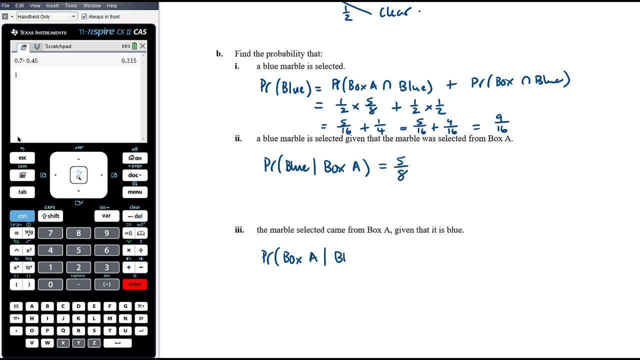 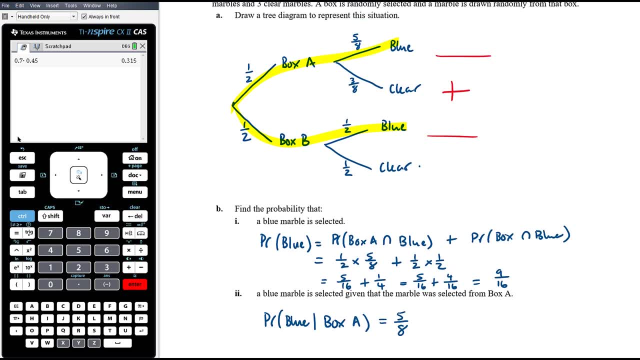 box A, given that we know that it's blue. Now, this is not sitting in the tree diagram, because the tree diagram isn't structured this way around. we've got boxes and then colours, so we've got the colours given the boxes. we don't have the boxes given the colours, So this is where we 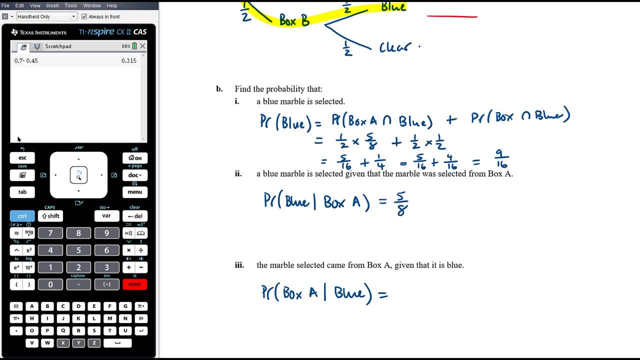 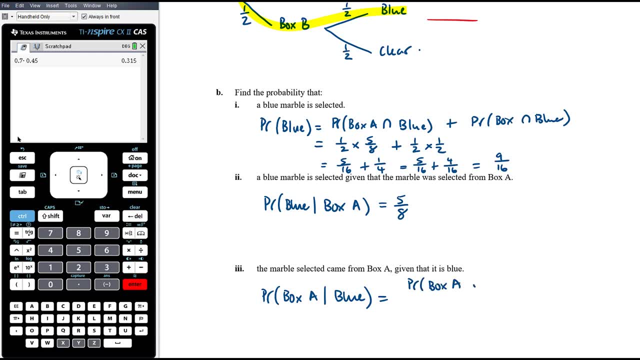 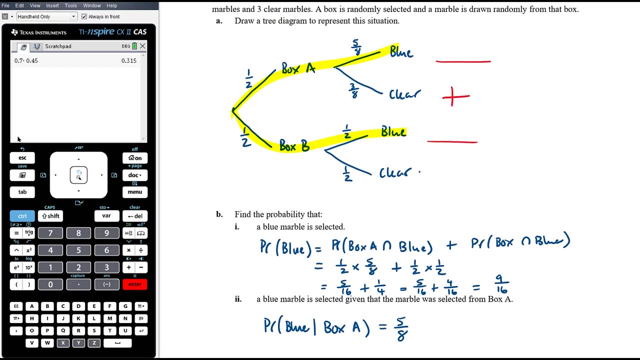 need to actually think a bit harder. we need to think about our. we need to think about our conditional probability, So that we know that for conditional probability it's the intersection of those two things. so box A and a blue marble Over the probability of getting a blue marble. So box A and a blue marble is one-half times three-eighths. 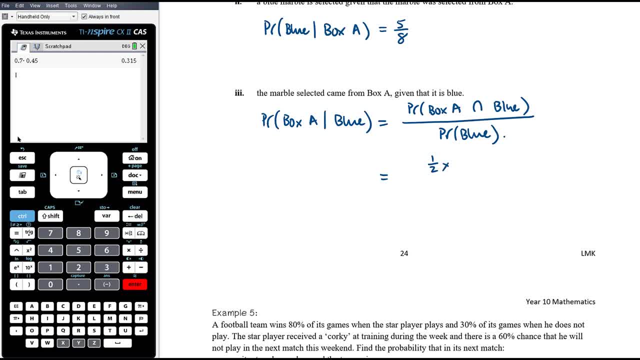 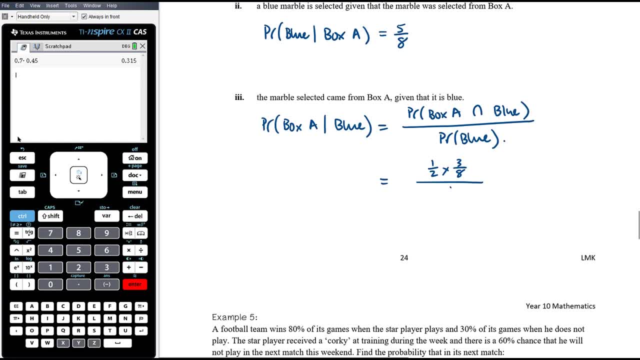 one-half times three-eighths divided by the probability of getting a blue marble, which we worked out in part B and B- part one sorry- which was nine-sixteenths. Okay, so the numerator there is three on sixteen. we're dividing that by nine on sixteen. 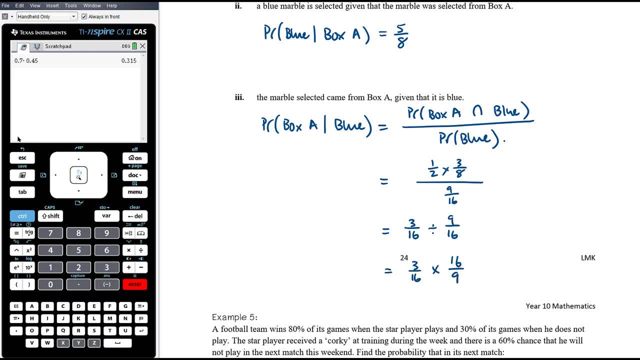 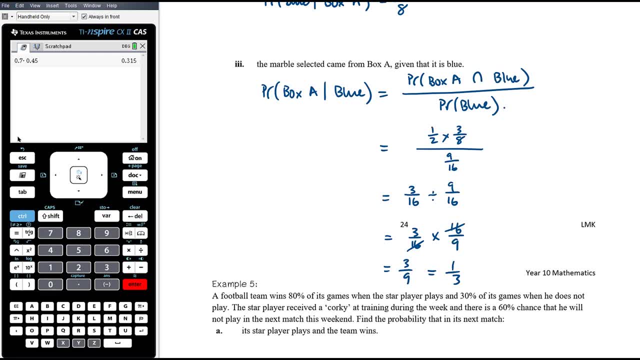 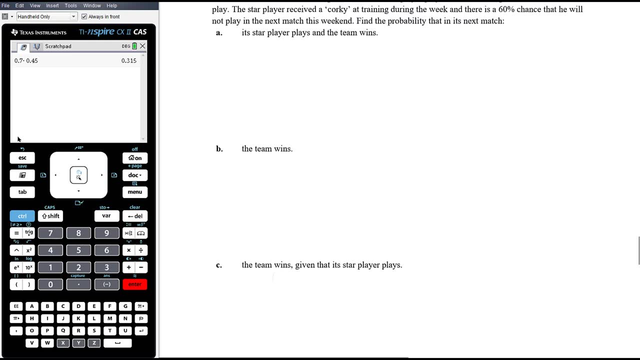 So that is three on sixteen times sixteen on nine. The sixteens are going to cancel down. we've got three on nine, which is one-third in simplest form. Okay, example five: I think it's the last one, Oh no, we've got two more. A football team wins eighty. 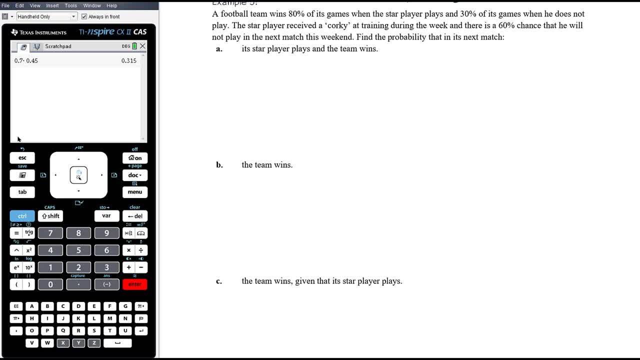 percent of its games when the star player plays and thirty percent of its games when he does not play. The star player received a corky at training during the week and there is a sixty percent chance that he will not play the next match this weekend. Find the probability that in its next. 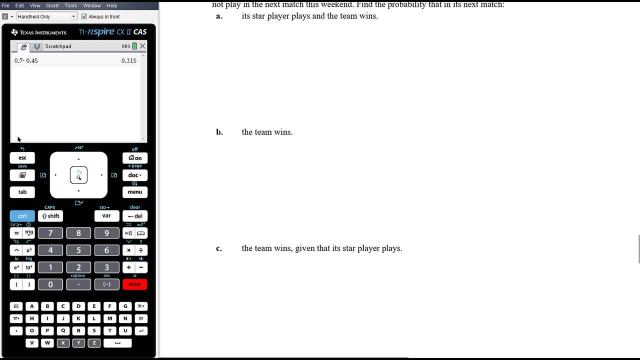 match. the star player plays and the team wins. The team wins. The team wins, given the star player plays. Its star player plays, given that the team wins. Okay, so we need to organize the information before we can calculate the probabilities. All right, so let's think about what happens. The 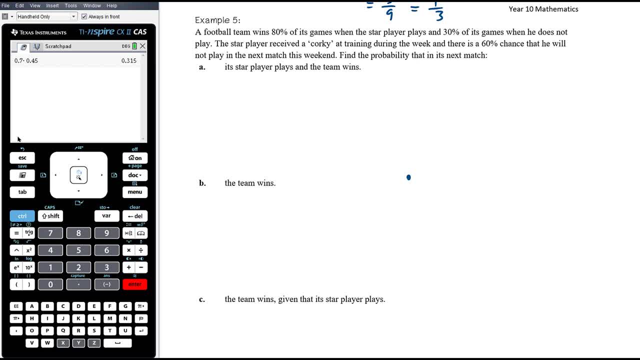 probability, that whether they win or not is dependent on whether or not the star player plays. So the first stage has got to be about whether the star plays. So the star plays, The star doesn't play. Okay, those are the two options, and then from there they either win or 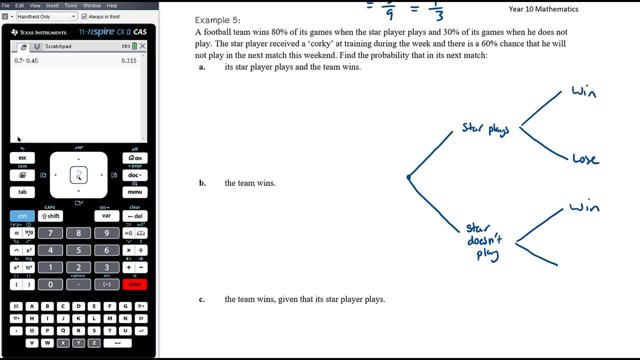 lose From there. they either win or lose. So again, it's about organizing your information so that then we can answer all the probability questions. It doesn't matter that the question doesn't say: draw a tree diagram. We need it in order to answer the questions. Okay, a football team wins. 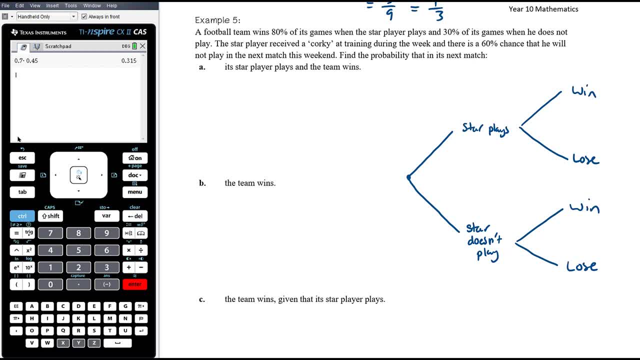 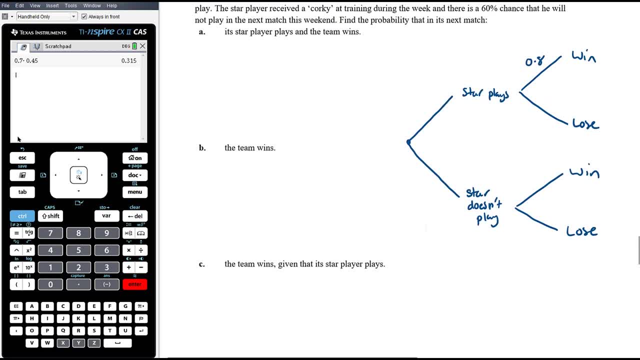 80% of its games. when the star player plays, The probability of winning, given that the star player plays, is 80%- That's that branch there- And wins 30% of its games when he does not play. So that's the probability of winning. given that the star player doesn't play, That's 0.3.. Now, 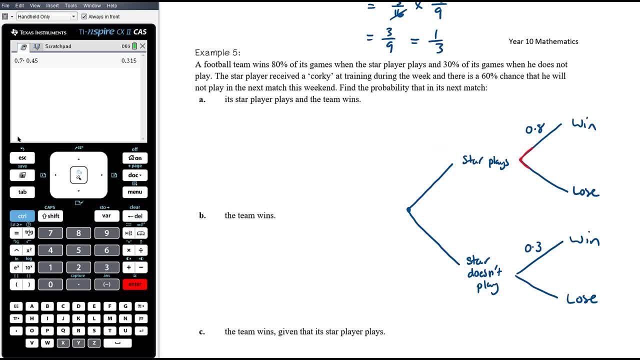 remember, all the probabilities that stem from the same point have to add to one, which means we can also work out: if there's an 80% chance of winning when the star plays, there's a 20% chance of losing. If there's a 30% chance of winning when the star plays, there's a 70%. 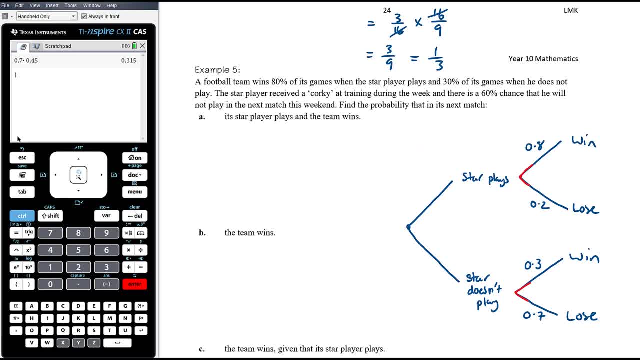 The star player received a core kit training during the week and there is a 60% chance that he will not play. So probability that you won't play is 60%. therefore a 40% chance that he will play. Okay, part A: The probability that the star player plays and the team wins- Probability that the star 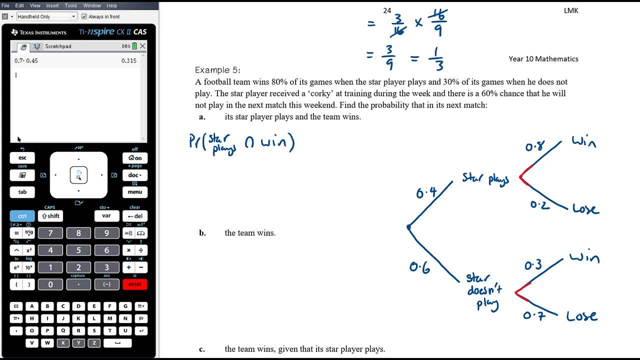 plays and the team wins. So that's simply going to be this branch here: 0.4 times 0.8.. Okay, 0.4 times 0.8.. 4 times 8 is 32. so 0.4 times 0.8 is 0.32.. The probability that the team wins: 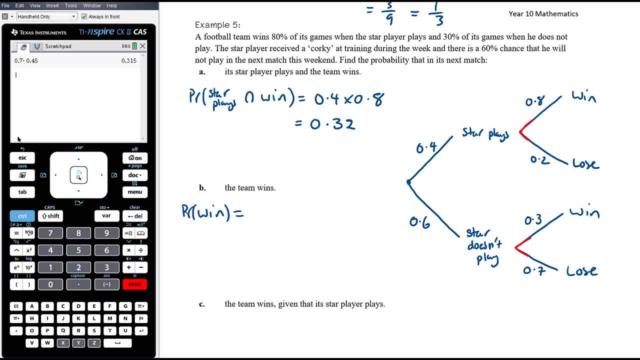 So there's two ways that they win: The star plays and they win, or the star doesn't play but they still win. Okay, so that's going to be 0.4 times 0.8, plus for the probability that the star plays and they win, plus so, or 0.6 times 0.3.. The star doesn't play, but they still win. 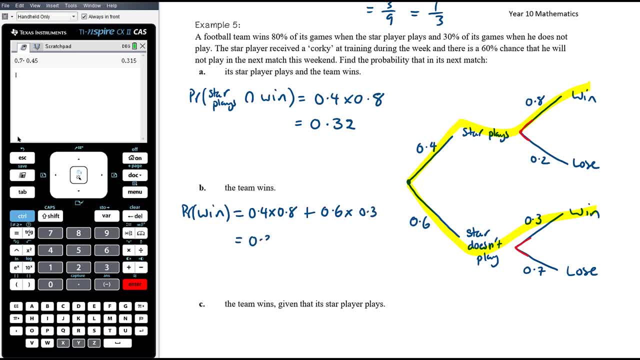 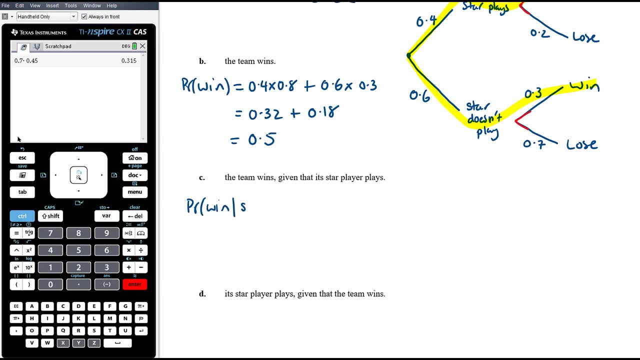 Sorry, 0.3.. So that's 0.32.. This is 0.18 and so that is 0.5.. So we have a 50% chance of winning Part C. Find the probability that the team wins, given that the star plays. 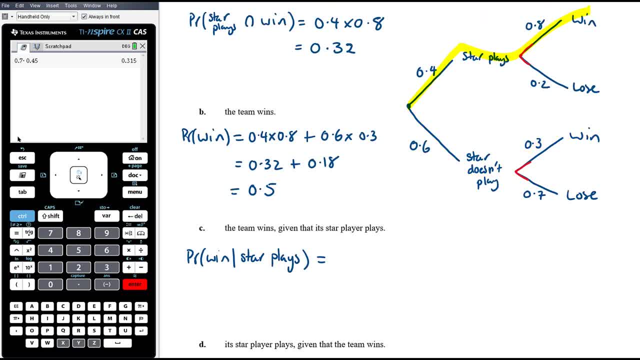 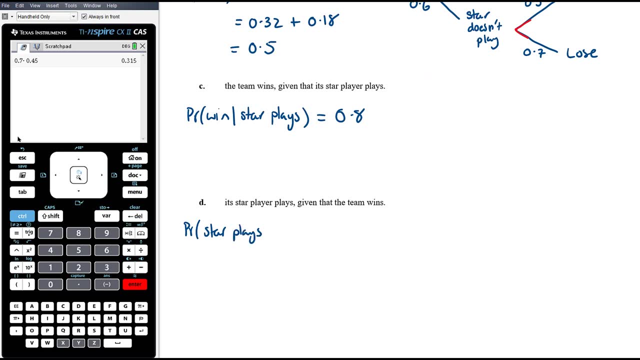 Okay, this one's actually sitting in the tree diagram. The team wins, given that the star plays. It's just that: 0.8.. The probability that the star plays, given that the team wins. Okay, so this is not how the tree diagram is set up, So we need to. 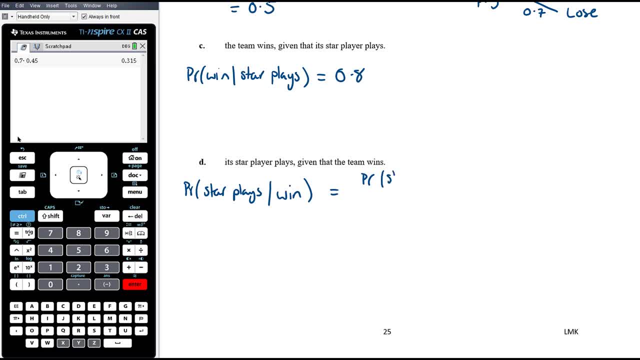 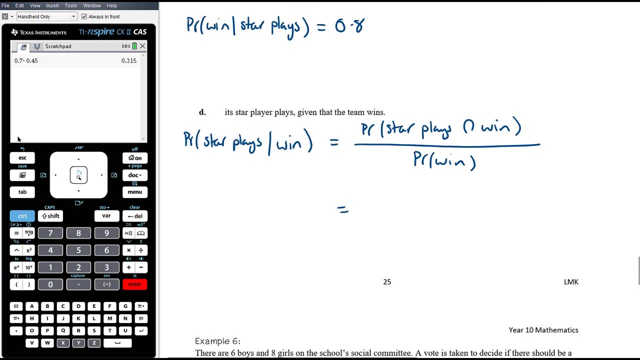 actually use our formula to calculate this. So we want the probability that the star plays and they win. so the intersection on the numerator over the probability that they win. Now we've actually calculated these two probabilities in parts A and B. So it's a 0.32 probability that the star plays and they win. 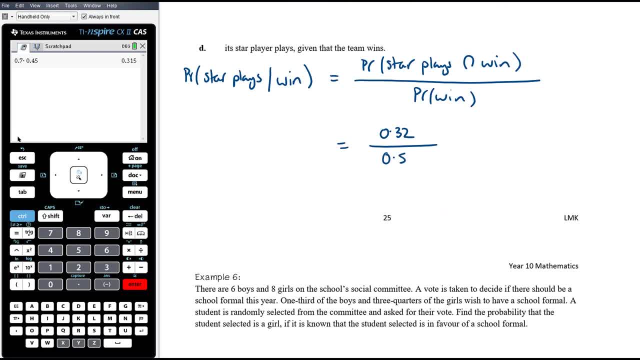 over, the probability that they win is 0.5.. Let's multiply the top and the bottom there by 100, so that's 32 over 50. And then we can simplify from there, so that is 16 on 25.. 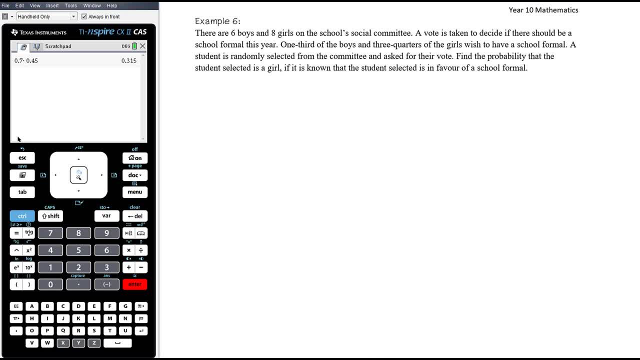 Okay, question 6, final example: There are 6 boys and 8 girls on the school's social committee. A vote is taken to decide if there should be a school formal this year. One third of the boys and three quarters of the girls wish to have a school formal. 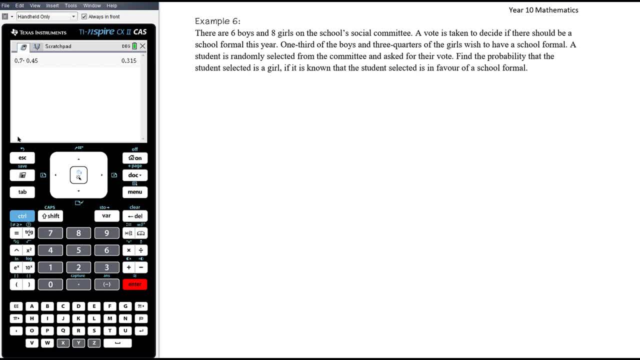 A student is randomly selected from the committee and asked for their vote. Find the probability that the student selected is a girl if it is known that the student selected is in favour of a school formal, Okay, so again, we want to organise the information. 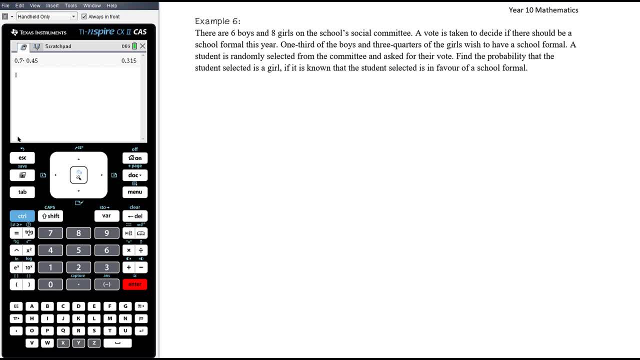 So we've got gender- boy or girl- and then we've got whether they are in favour or not in favour of the school formal. Okay, so let's set that up: Boy, girl. I'm just going to make for or against the formal. 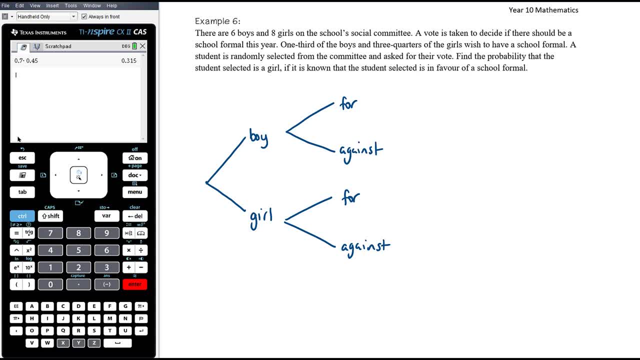 For or against the formal Okay, there are 6 boys and 8 girls on the social committee, So that means there's a committee of 14, 6 out of 14, so that's 3 out of 7- are boys. 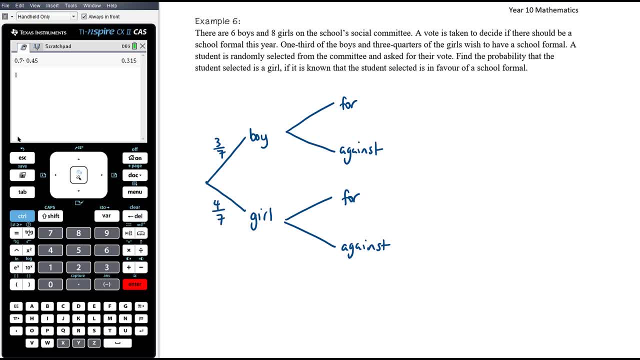 and 8 out of 14,, so that is 4 out of 14.. So that means there's a committee of 14, 6 out of 14,, so that's 3 out of 7, are boys and 8 out of 14,, so that's 4 out of 14, so that's 4 out of 7 are girls. 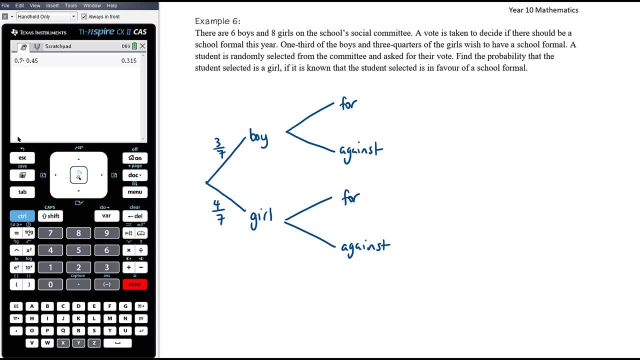 1 third of the boys are for the formal, So probability being for the formal, given that you're a boy, is a third, which means 2 thirds of them are against it And 3 quarters of the girls are for the formal. 1 quarter is against it. 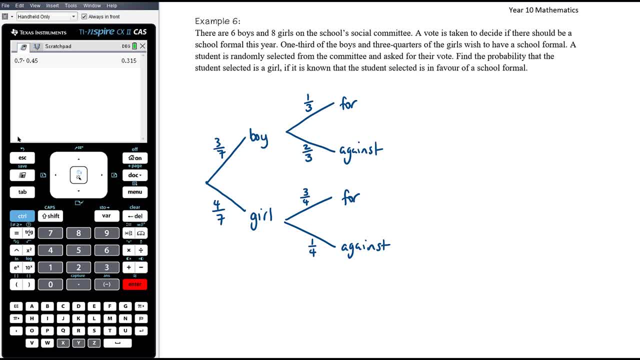 Okay, we want to find the probability that the student selected is a girl. if it is known that they are in favour of a formal, This is a conditional probability, Given that they are in favour of a formal. Okay, so we want to know the probability that someone is a girl. 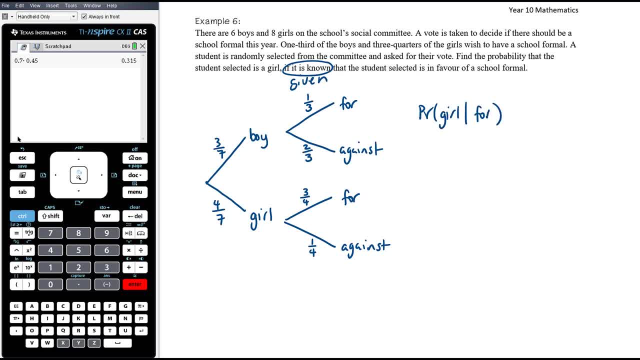 given that they are for the formal, They're in favour of the formal. Okay, so that means again, the diagram isn't set up like this If it was asking us for the probability that they're for the formal, given that they're a girl. 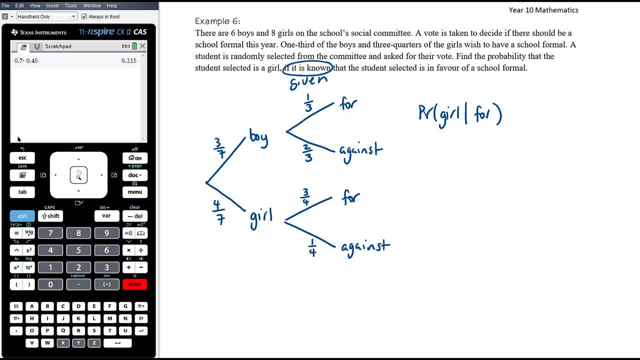 that would be just here, sitting here 3 quarters, But it's set up. the tree diagram is set up the other way around and we can't change the tree diagram around. We have to just calculate our conditional probability using our formal. 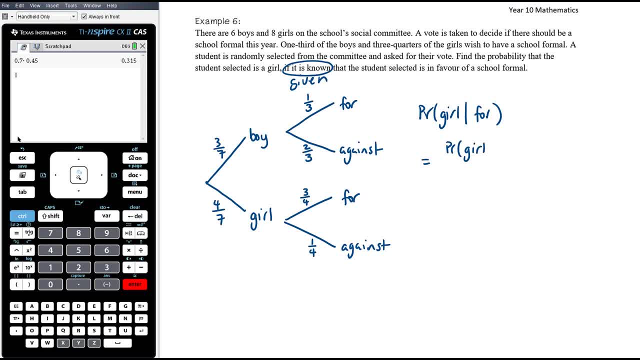 So we want the probability of being a girl and for the formal over the probability of being for the formal. Okay, so girl and for is 4 sevenths times 3 quarters, divided by being for the formal. there's two ways that that can happen. 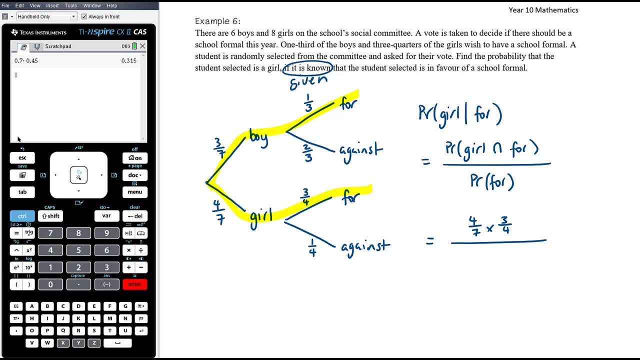 You can be a boy that's for the formal or a girl that's for the formal. So essentially it's the green path. try and not hide the yellow. the green path divided by the total of the yellow path: Okay, so probability of 4 is 3 sevenths times a third. 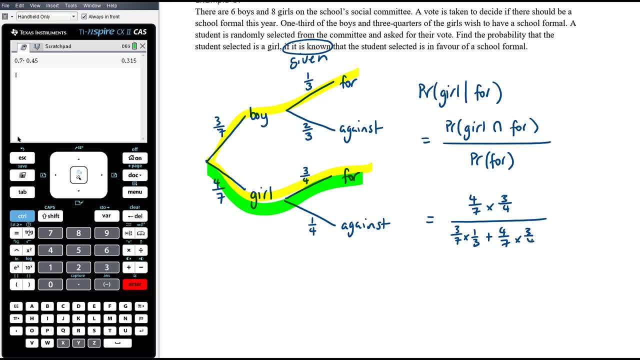 or 4 sevenths times 3 quarters. Okay, so let's simplify: 4 sevenths times 3 quarters is 3 sevenths. This is again the 3's cancel there. so that's 1 seventh plus.